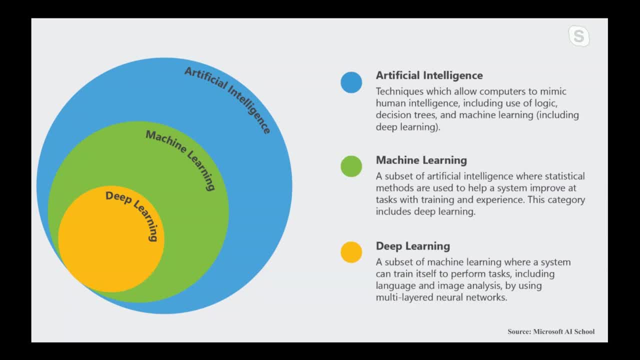 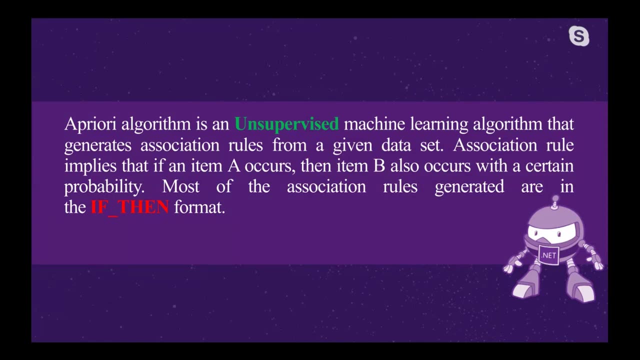 also a part of artificial intelligence. so here today, our main topic is machine learning. we are talking about a pretty algorithm, which is a machine learning algorithm. so what is a pretty algorithm? a pretty algorithm is an unsupervised machine learning algorithm that generates association rules from the. 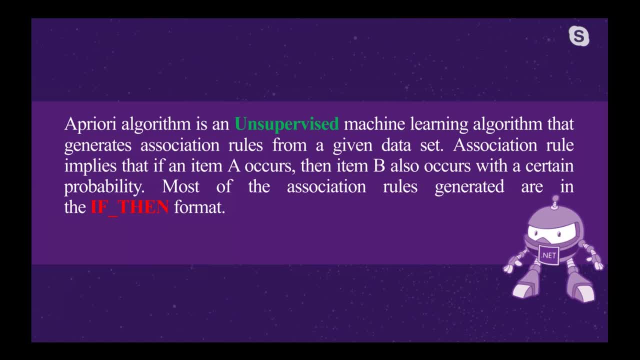 given data association rule implies that if an item A occurs, then item B also occurs with a certain probability. most of the association rules generated are in the if-then format. so here we see that there is a word which is unsupervised. what is unsupervised? unsupervised means unlabeled data when any machine learning. 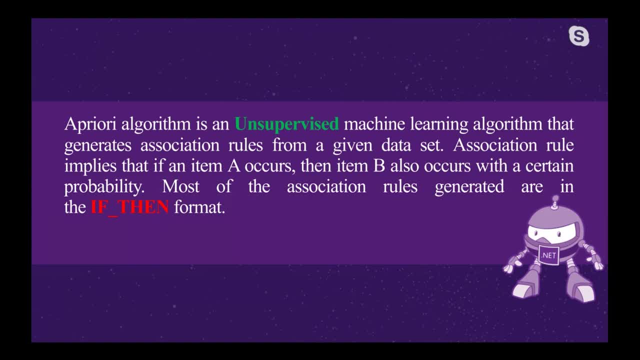 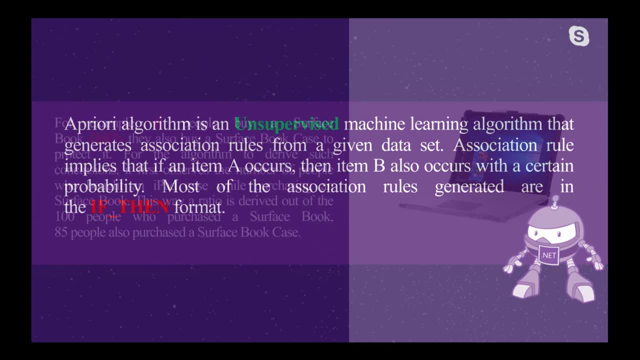 model learns a new machine learning model. it is unsupervised, and unsupervised machine learning is learned from unlabeled data. this is we called unsupervised machine learning, unsupervised learning. so going to our next slide, for example, if people buy a surface book, then they also buy a. 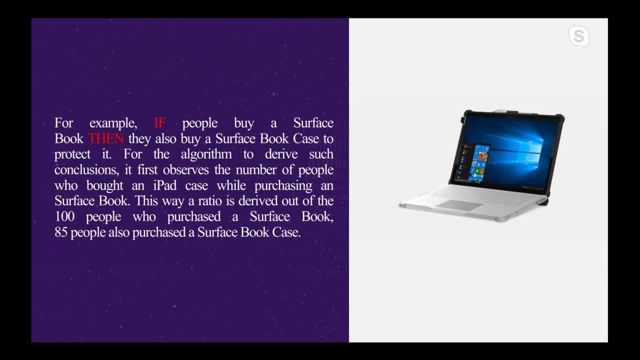 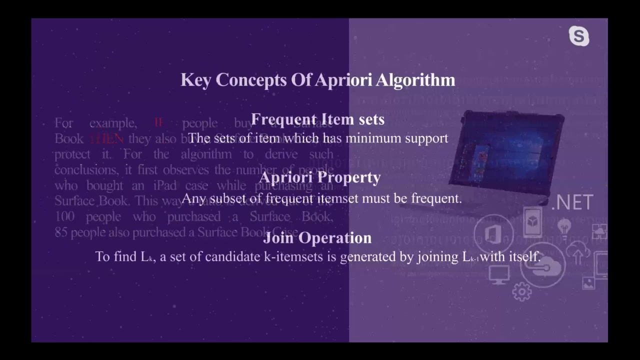 surface book case to protect it. for the algorithm to derive such conclusions, it first observes the number of people who brought an iPad case while purchasing a surface book. this way, a ratio is derived out of the hundred people who purchased a surface book. eighty-five people also purchase the surface book case. next slide. so there are some three key. 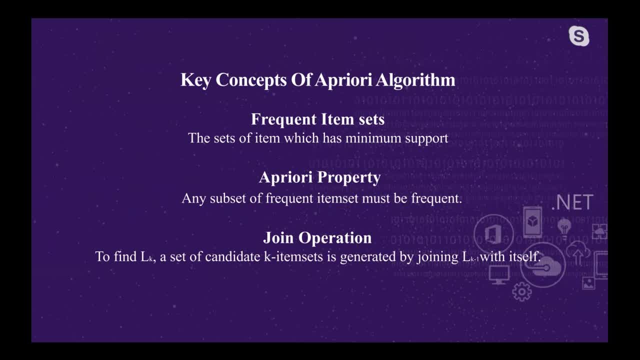 concepts of a pretty algorithm which is frequent items at a pretty property and joint opposition. what is frequent acting, said frequent headset, is a set of item which is medium support. what is a pretty property after the property is a subset of infrequent items. that which is must be frequent. 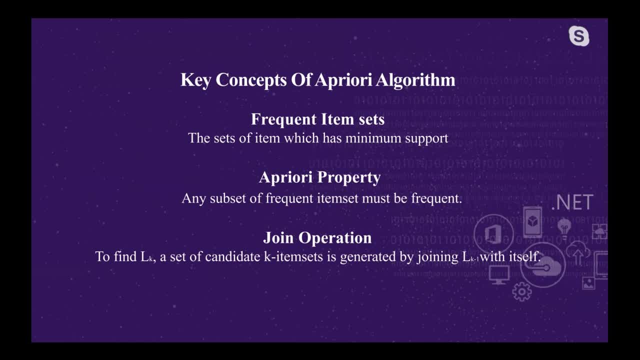 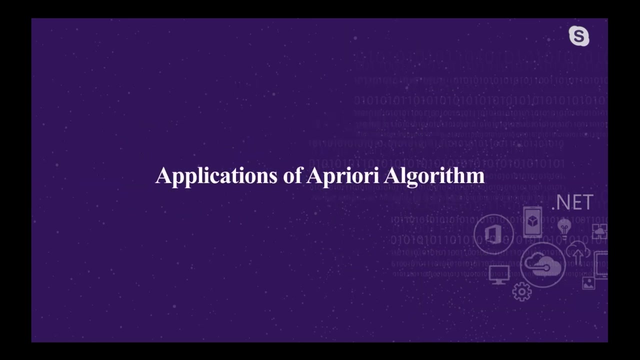 join operation. to find join operation means when One or two items that create a new item set, So this is we called join operation. suppose to find LK case: a set of candidate K item set is generated by joining LK minus one with itself. Applications of a pretty algorithm. 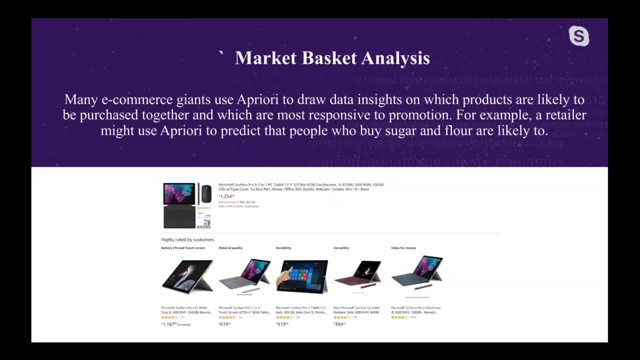 So market basket analysis is the one of the most common applications of a period. with them, many e-commerce giants use a pretty to draw data insights on which products are likely to be purchased together and Which are most responsive to promotion. For example, a retailer might use a pretty to predict 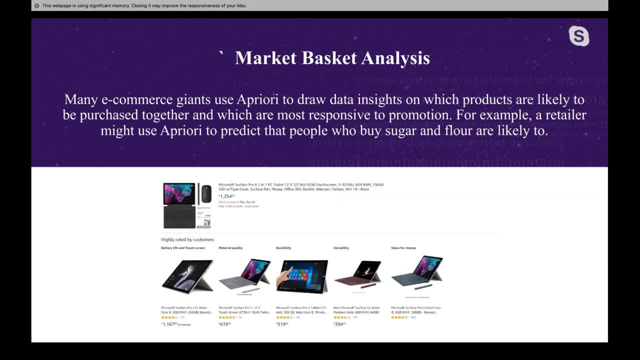 People who buy sugar and flour are likely to. in a picture We see that when we search ecommerce site market basket analysis For buying a Microsoft Surface Pro, So we see that there are other similar product like that. So in this picture we see that system show other. 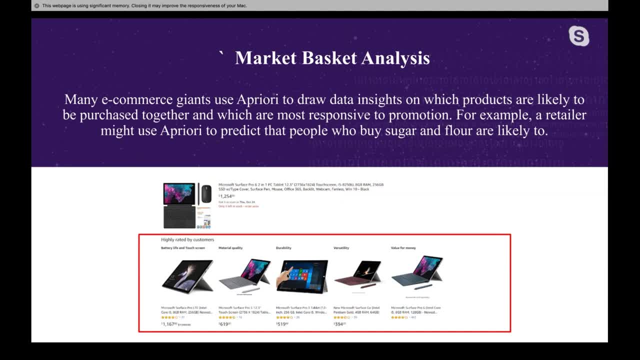 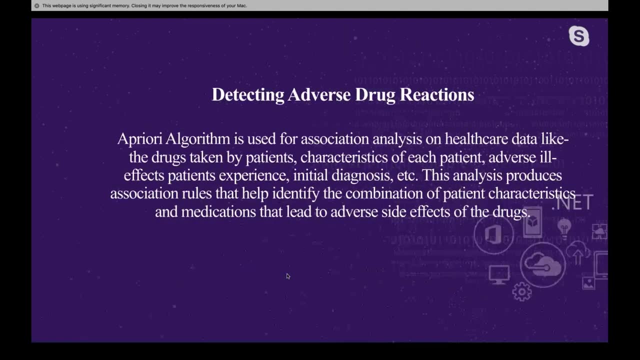 Similar Microsoft Surface Pro or surface book or something like that. So this is called and this is here. actually a pretty algorithm works Here. a pretty algorithm create these items set and show the customer this product. So another application of a pretty algorithm is Detecting adverse drug reactions. a pretty algorithm is used for association analysis on healthcare data, like the drugs taken by patients. 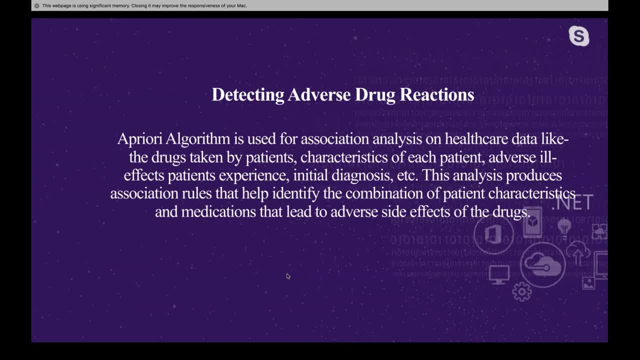 characteristics of each patient, adverse ill-effects, patient experience, initial diagnosis, Etc. This analysis produces a session rules that help identify the combination of patient characteristics and medications that lead to adverse side effect of the drugs. So actually here a pretty algorithm: create rules for the patients. 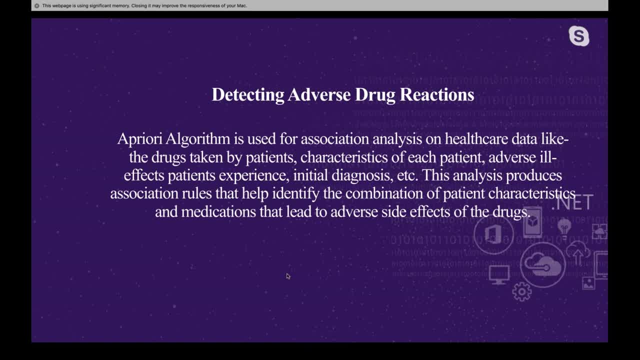 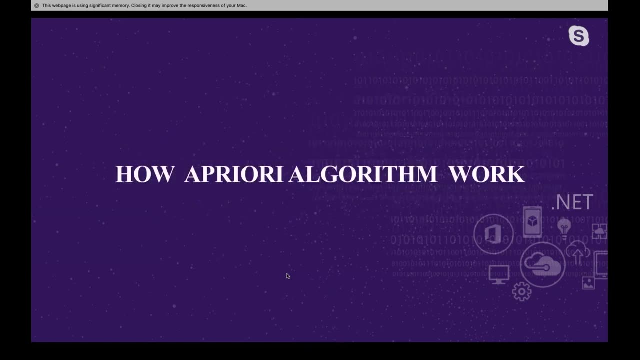 create rules from the Drugs which is used with patients. What is a side effect of these drugs? How actually works for the patient of these drugs. So here actually a pretty algorithm work. So now we are diving into how actually a pretty algorithm work, how it works. 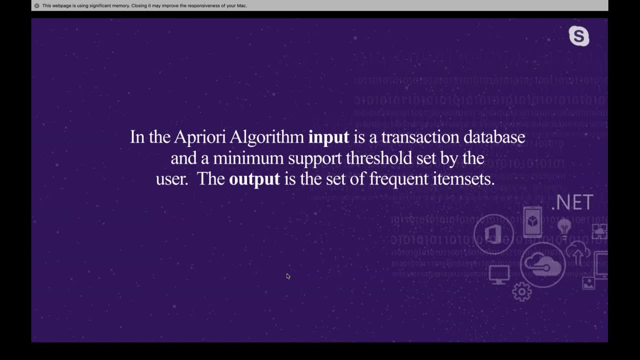 before studying that, We need to know that what is input and what is output in a pretty algorithm. In the algorithm, input is a transaction database and a minimum support threshold set by the users. and what is output? output is a frequent at a set of. So actually here. 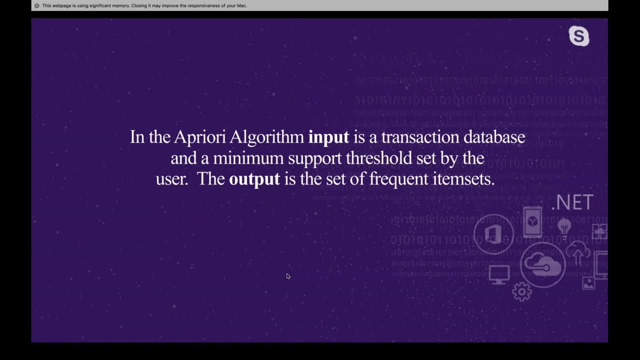 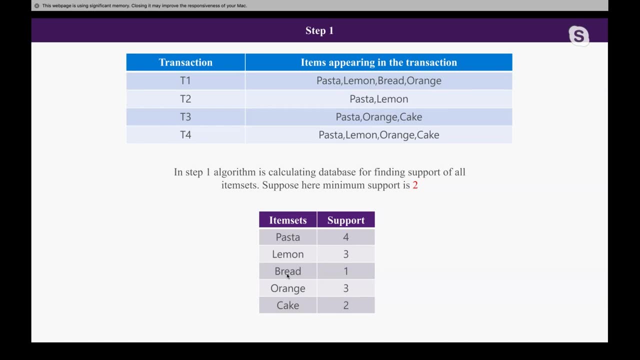 Input is transition database and output is frequent at insert. So in our first step we see a table Where there are four transaction and items that are Pasta, lemon, bread and orange. so we see that each transaction Have a the different item set. We see that in transition one There are four items set. in transition two There are two items set. three have 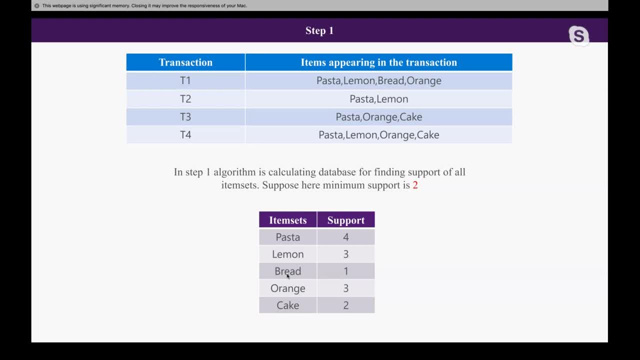 three items set and four have four items set. so in our item set we see that For pasta our Support is four, for lemon it is three, for bread It is one, for orange it is three and for cake it is two, But here our minimum support is two. So in this step we need to find 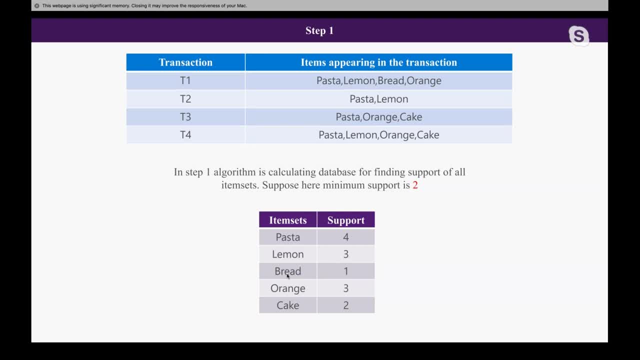 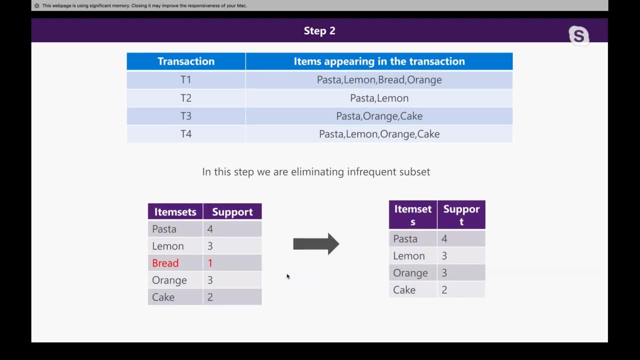 The item set which is below our minimum support. so here we see that bread is our, bread is a bread, item set as medium support is lower than our medium support. our medium support is two and here bread is a bread Support is one. so we need to cut down this item set and create a new table. 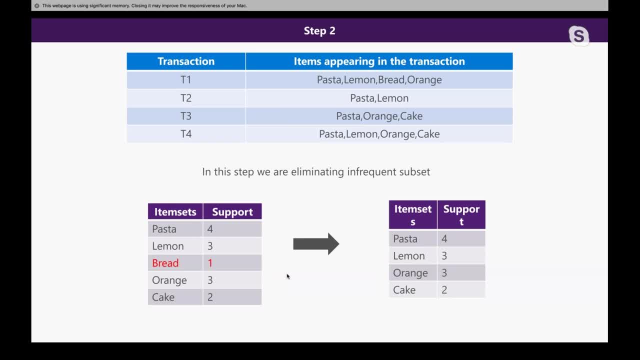 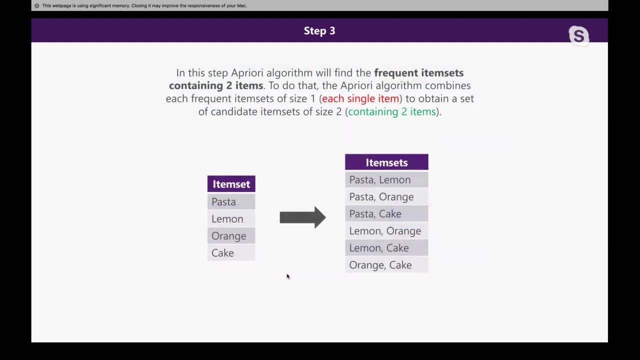 So here we see that For new item set we got pasta, lemon, orange and cake and Each item set and a support value is equal to or greater than our minimum support in this step. we see that Each item set In this step- April grade them- will find a frequently return set containing two items. 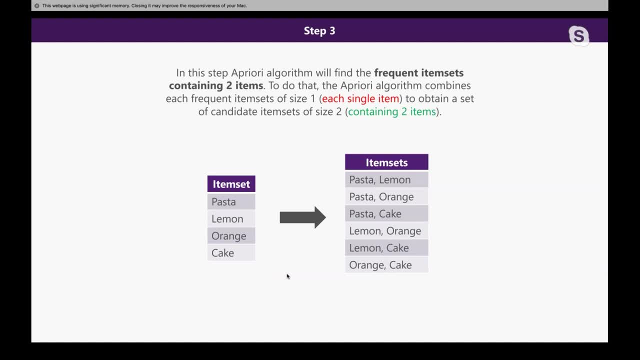 To do that, the April algorithm combines each frequent at insert of size one, each single item Really, to obtain a set of candidate item set of size two, continuing two items. so here we see that from size one item set two, we are creating such a item set from size two item set. there we see that there are six item set in our 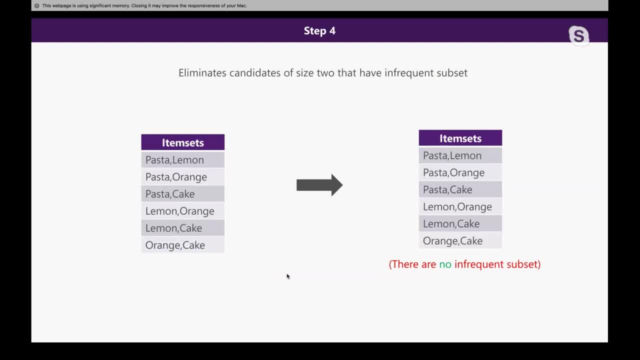 next step. we see that there are. we need to find it. is there any infrequent item set or not? so we see that there is no infrequent item set. so what is infrequent item set? I told you, you know, in my previous slide. so actually, influent item set is the those item set which have a infrequent subset. so there, 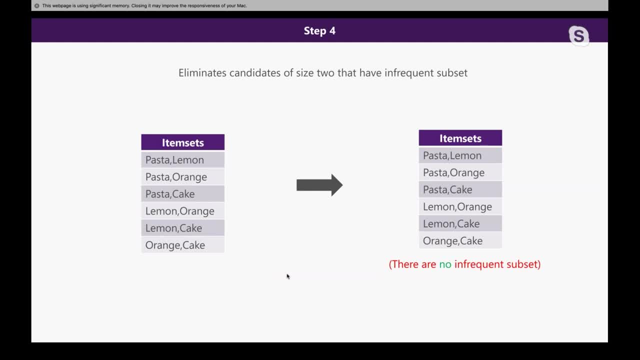 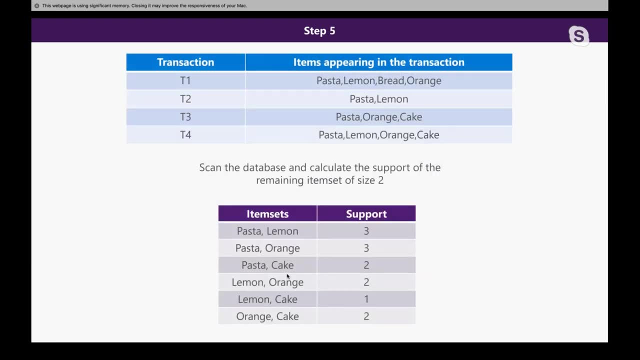 is no infrequent subset of this item set. so there are no infrequent item set. in my step 5 we see that we again need to we we again need to calculate which item set support value is less than our medium support. so here we see that. 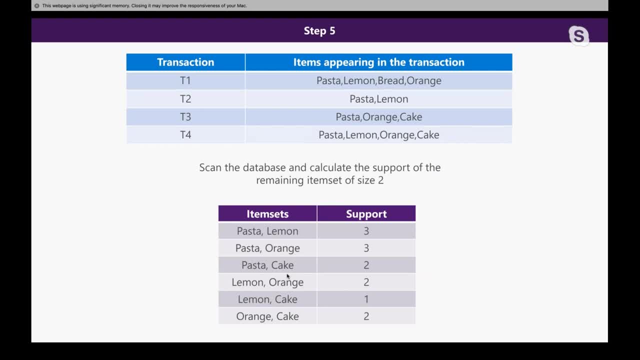 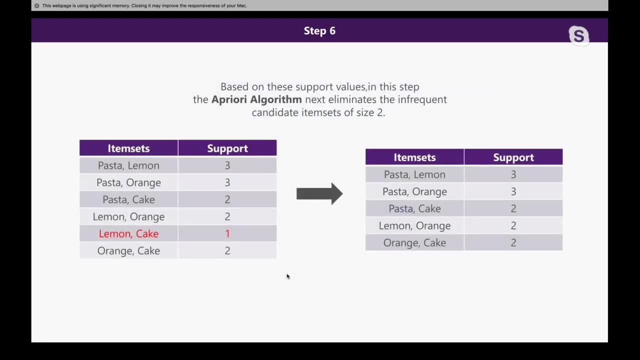 lemon and cake is lemon and cake because support value is less than our minimum support, which is one. so we need to cut down this uh, lemon and cake and create a new item set table. so here we see that, uh, we got pasta lemon, where support value is three, pasta orange, where supper value is three. also, pasta cake is four, is two. 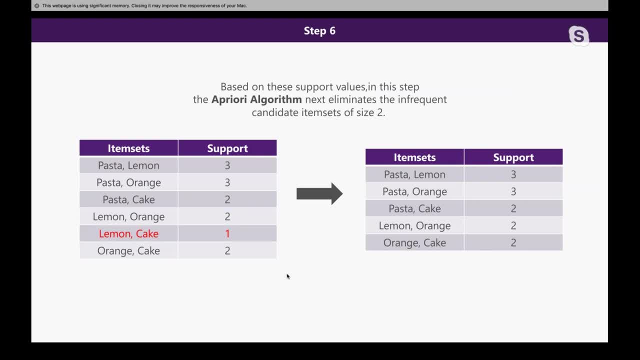 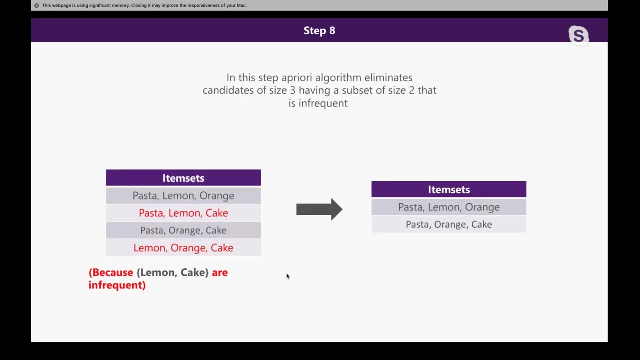 sorry, uh, lemon orange is two and orange cake it is two. so here we are, creating support value, we are taking those support value, which medium which is equal to or greater than our minimum support in this step, in step eight, in this step, we need to find also again: uh, is there any infrequent? 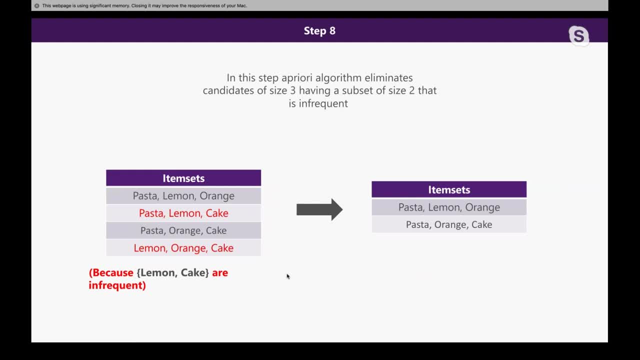 set or not. so here we see that now in this time we got two infrequent subset, so which is pasta, lemon cake and lemon orange cake, because here lemon and cake are infrequent, so we need to again, uh, cut this item set and create a new item set table. 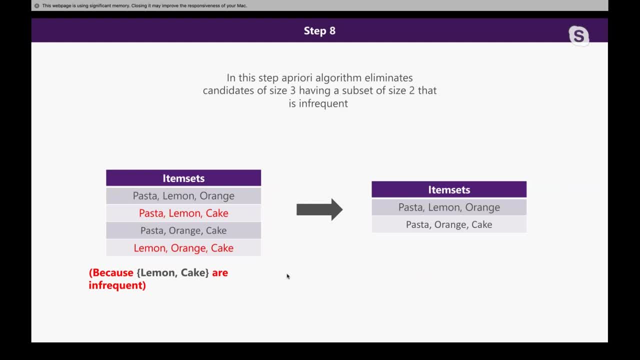 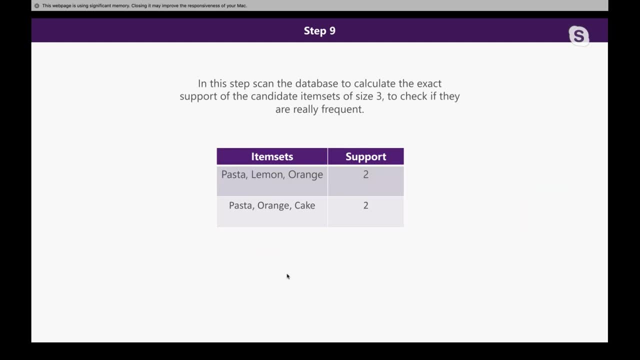 so from here we got two item set, which is pasta lemon orange and pasta orange cake. so in this step, uh, we again scan the database to calculate the exact support of the candidate item set of size three, to check if they are really frequent. so we see that, uh, our both item set. 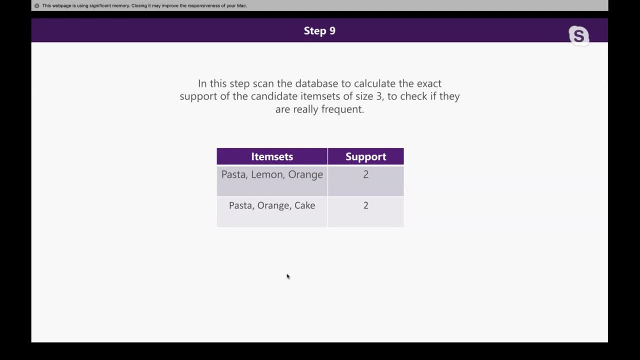 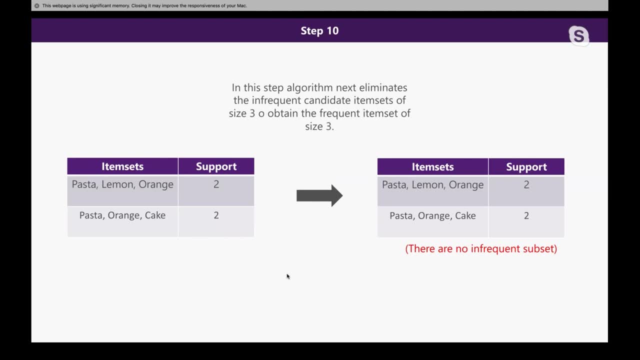 support value is equal to our medium support, which is two. so there is no problem in this step. we again see that, uh, is there in any infrequency subset or not? so here we see that there are no influence subset because there are no item set, which is infrequent. so we are taking two of this item set. 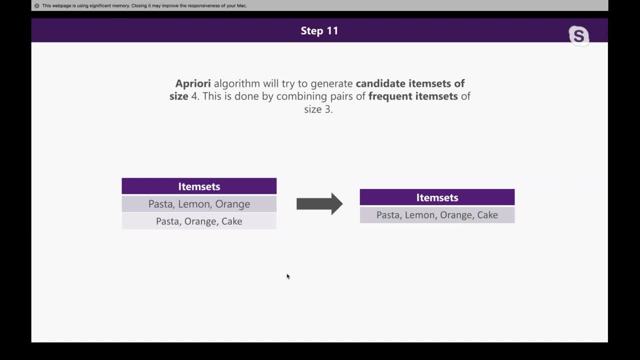 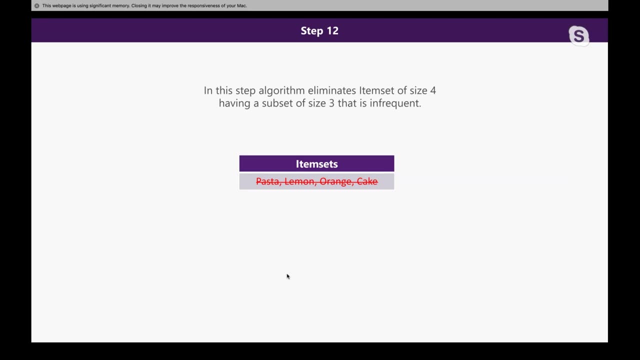 so now in this uh three size three item set, we are creating now uh size four item set which is pasta, lemon, orange and cake. so now we see that uh algorithm eliminates uh item set of size four having a size, uh subset of size three, because that is infrequent, because we see that uh, there is a lemon and cake. 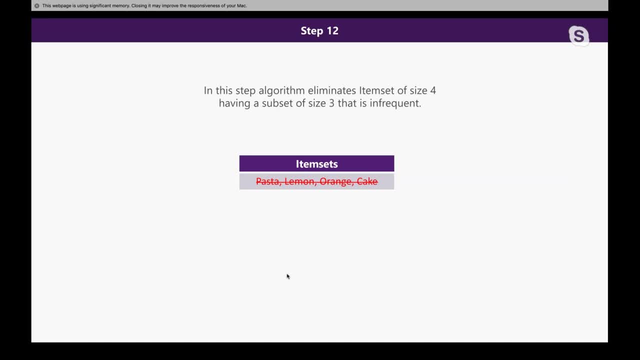 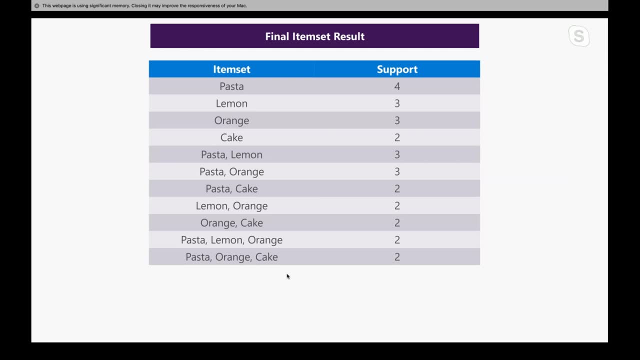 so we know that a lemon and cake is, uh, infrequent subset, so we need to cut down this item set. so now we got that there are 11 item set. this is our main final item set result. so here we see that for pasta their support value is four, for lemon it is three for orange, three for cake is true pasta and 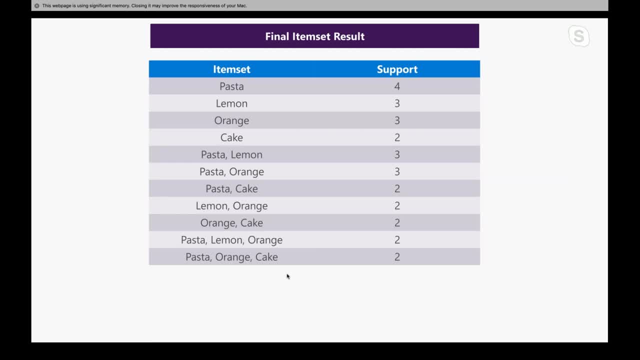 lemon and pasta and orange. both are three: pasta and cake- lemon- orange- orange cake, pasta lemon- orange and pasta- orange cake. they are also two. so here we see that. uh, each item says support value is equal to or greater than our minimum support. so there is no problem. so this is our. 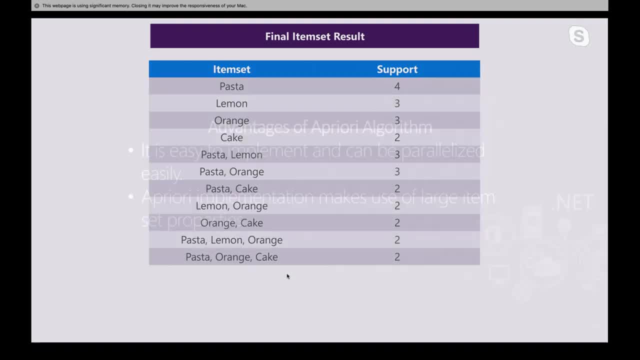 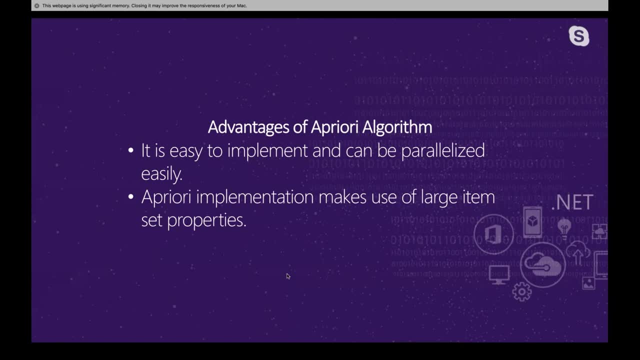 final item set. so, uh, what is the advantages of april algorithm? so actually it is uh implement- is it is easy to implement and can be paralyzed easily after the implementation? make use of large item set properties. so we see that when, uh, we are using uh april algorithm in e-commerce site or 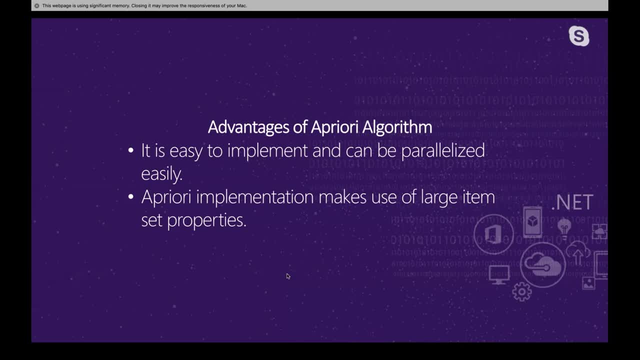 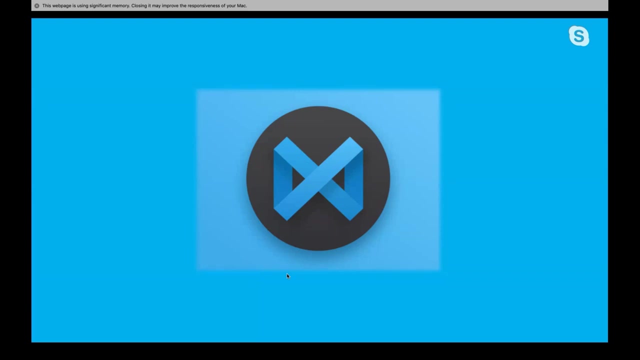 something like that. we can easily implement it and it can. it can be paralyzed easily rather than other machine learning algorithm and it is perfect for the association rule based machine learning model. now we see a simple uh applications, uh on the on based on this uh april algorithm. 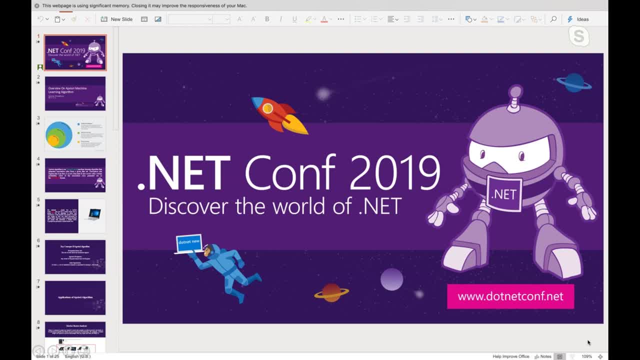 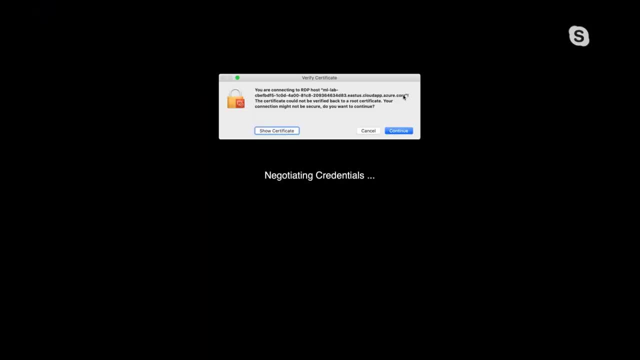 so it says that if we are using the application, you should have four different items. um, uh, so we will use the application. you can easily apply a method you would like to apply here and in this example, we are gonna show a path. by the way, the content of the content is, in fact, a graph, so it will be a graph of the real value to no. 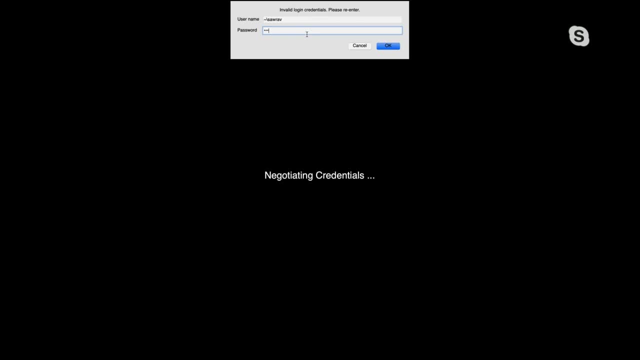 matter what the value of the thing is there, and it will tell you how much is it less than the value of the value of the item. so we are going to go ahead and apply this path of no matter how much you can do the target data to this query and it will tell you how much. 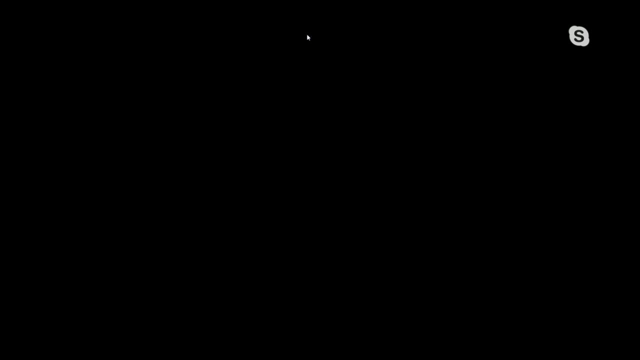 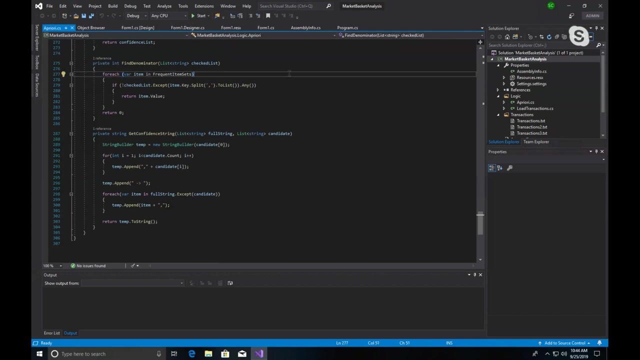 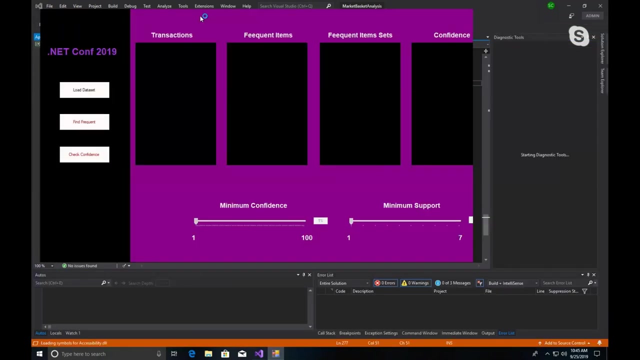 the value of the item is, and then the quantifier will tell it how much it is, and if you will add other. so here we see that this is our applications, this is our main algorithm. so if we run our applications so that, so we say that there is a four balls, which is one for transition. 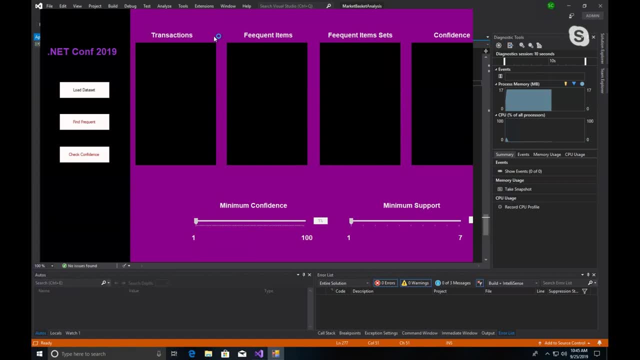 frequent item set. another and another one is frequent item sets. and last one is confidence. so here we see that there is a um, there is a option for our minimum confidence. so here we select our medium confidence is two, sorry, um, here we select our medium confidence: 60 percent. 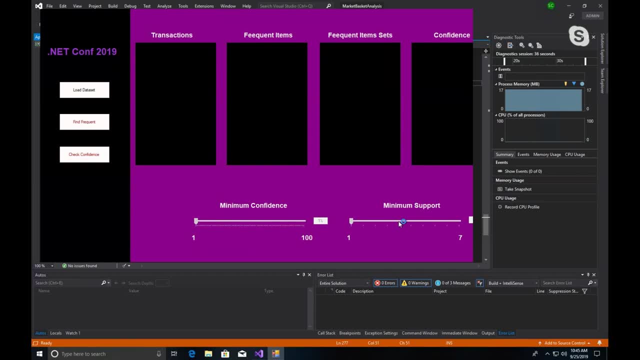 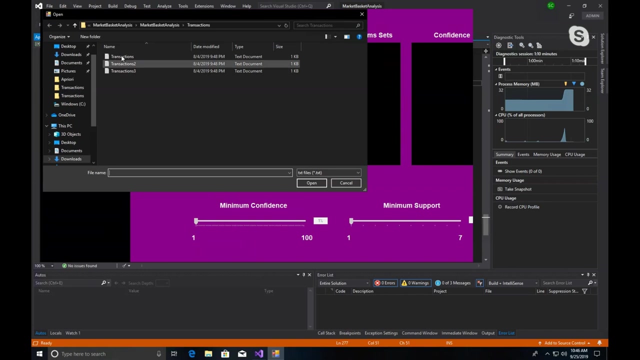 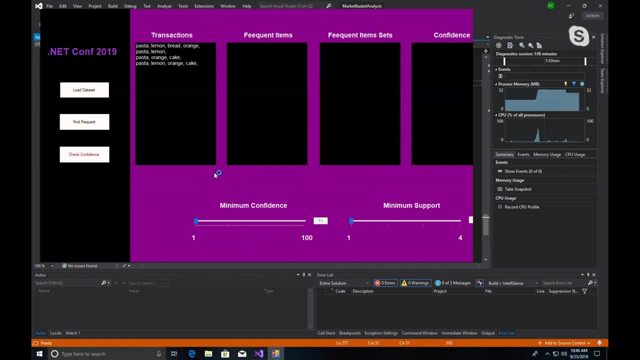 and also we are selecting our minimum confidence. uh, two, medium support is two. oh, it's a connection problem. so, um, here we are, load our transition data set. so we see that. uh, our transaction, that is, uh show in the transition box which is pasta, lemon bread and pasta, um, lemon pasta, orange cake and pasta, lemon, orange cake. so, uh, now we see that, um. 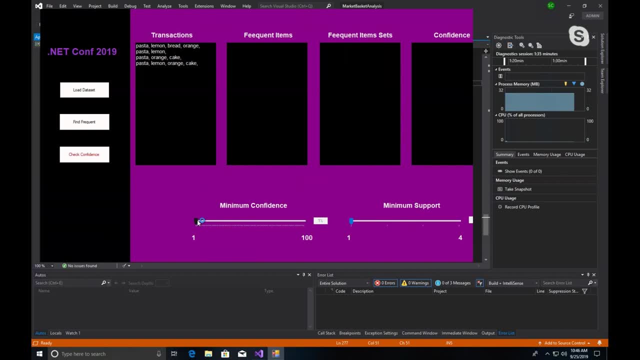 we can see that uh, um, and 저희가 are going to select uh this minimum. so if we uh change our minimum confidence into 61 percent and our minimum support- we change, our genial support- is two. so, uh, now we are find our frequent items. 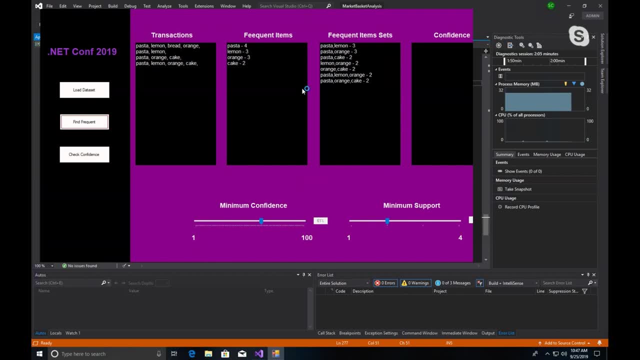 which is pasta, lemon, orange and cake, and each item set value is uh. item set uh support value is equal to or greater than our minimum support, which see before in our slide, and now we see that we check our confidence. so this is our main association rules, uh for this item set uh transaction. so here we see that. 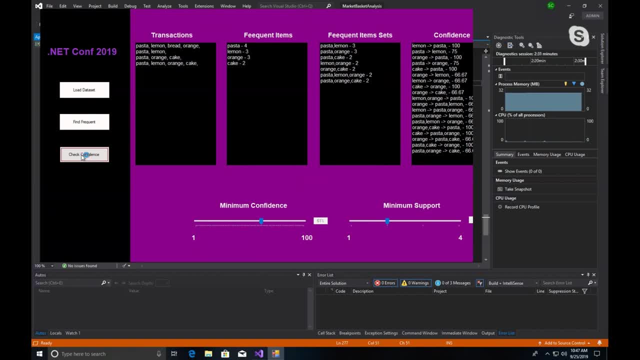 in confidence section um each item set confidence section is greater than equal to 60 percent. so if we change our confidence value, which is uh 46 percent, so if we again check our confidence, so here we see that there are many other more confidence um association rules i can set. so which is uh past the orange cake. 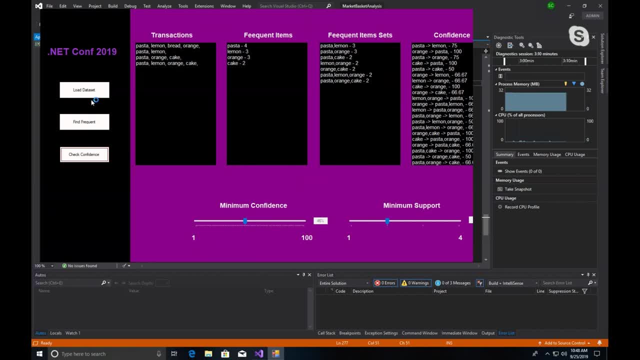 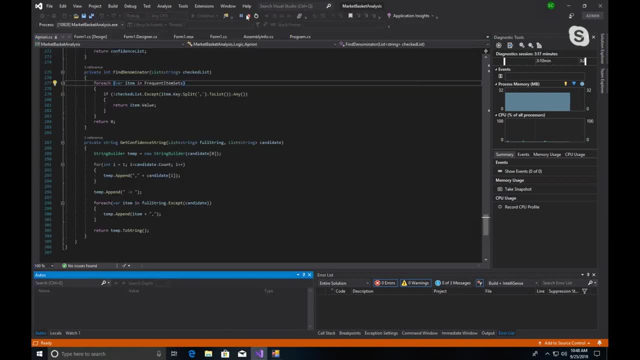 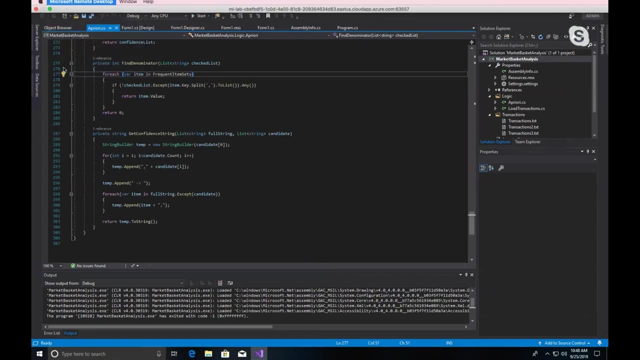 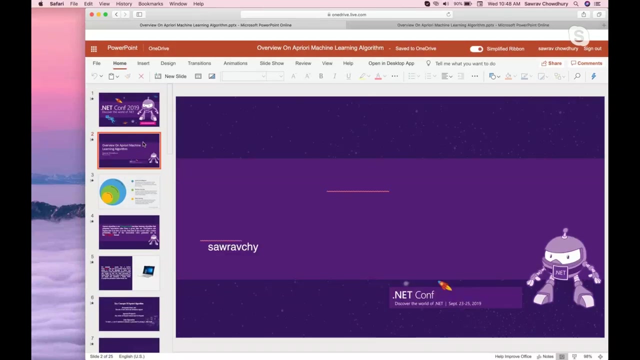 which is 50. uh, minimum confidence is 50 percent. so this is our application. so, uh, in our uh whole session we learned that, um, what is actually a critical freedom? uh, how actually it works. uh, which kind of uh platform is perfect for appropriate rhythm? we see, 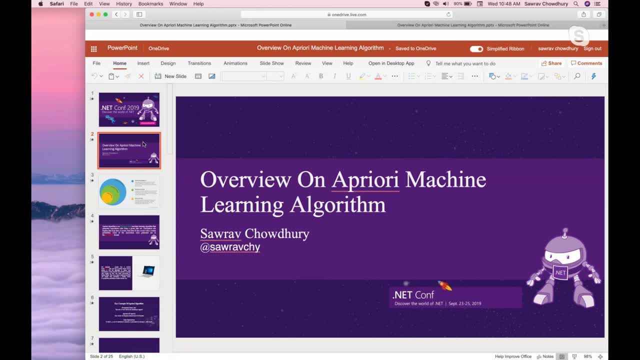 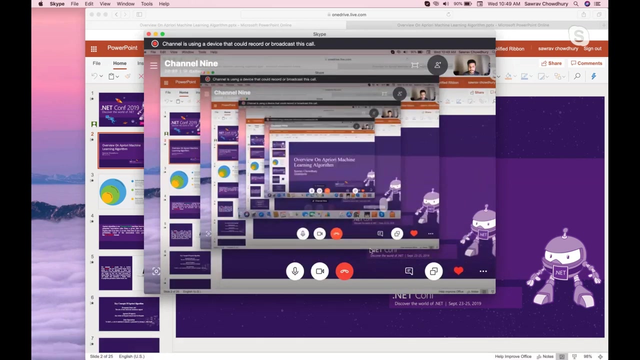 that, uh, most of the cases are e-commerce sites for creating association rules, which is perfect for this algorithm. so we see that, uh, most of the cases are e-commerce sites for creating association. so, so, so you keep recording, um, so a fun, and i think we can karen. 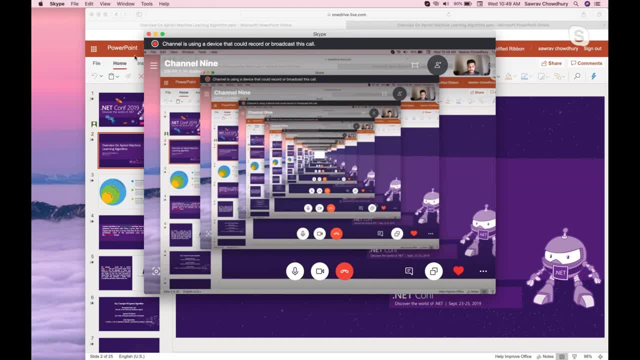 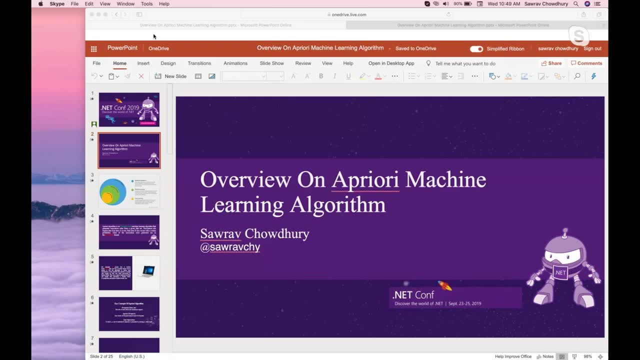 we can, we can really, you know um, can you? yeah, everybody on the chat, do you guys hear the echo anymore? yep, we still got echo, all right, sweet echo, all the things. goodness, thank you for that. for sounding, yes, oh, sounds great. no echo, no, echo, sweet, thank you. I thought there was an. 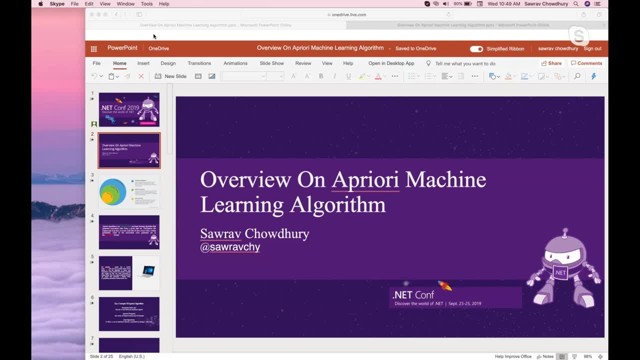 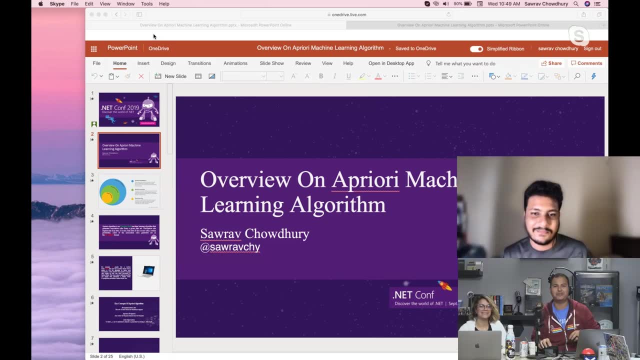 echo- perfect. thank you so much, sir Rob. I don't think we got any questions. so yeah, I mean the epic win here. I'm going to switch this over here to the Q&A so we both see each other. the epic win of the day is that we don't have an echo and we